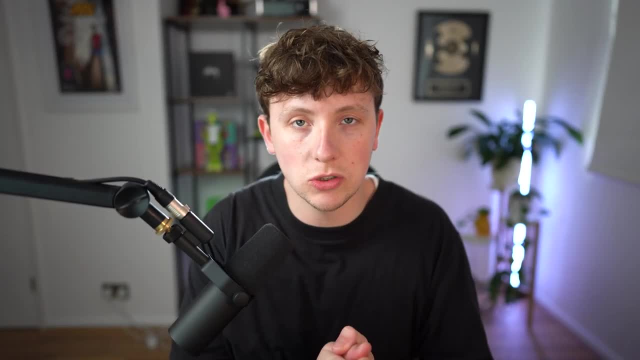 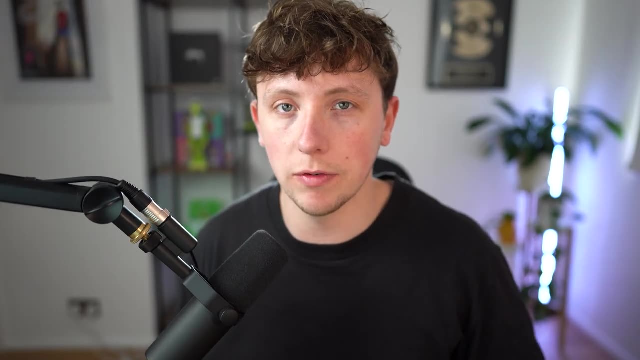 automate certain parts and to help us make this process super, super simple. This literally applies with every single business when it comes to social media. Follow along and see how you can use these tools for yourself. First things first. we're going to want to be able to create content. 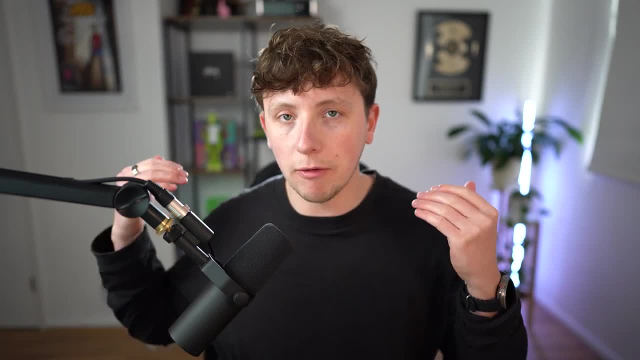 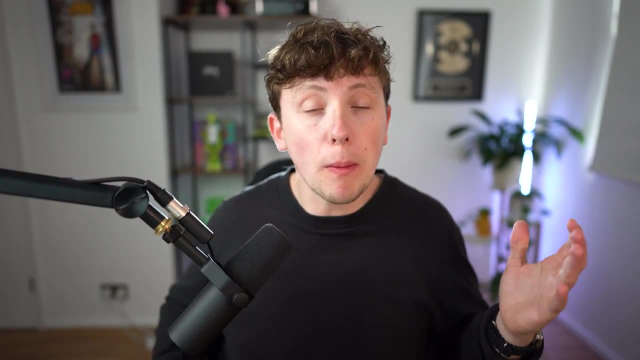 for our business. We need to be coming up with new ideas and we need to keep our feed exciting, with exciting imagery and exciting videos that get our customers engaging and clicking through to our site. Previously, we probably would have had to pay a content creator or a designer to do this. 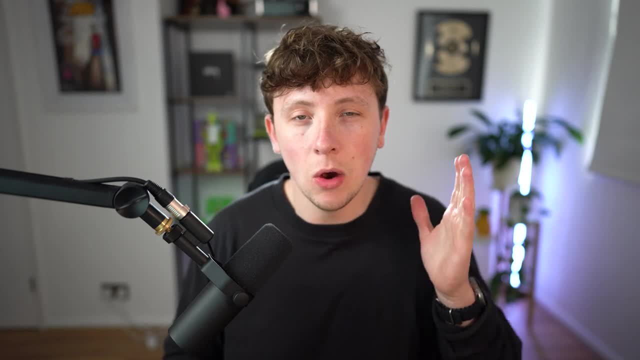 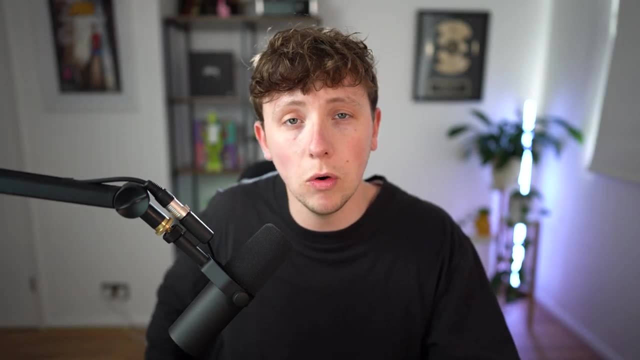 for us, and it gets very, very expensive and very difficult to maintain when there's not a ton of money coming in from it. Now, some of you may have heard of Canva and you've probably used it for your businesses or your social media before. but we now have access to Canva and their AI. 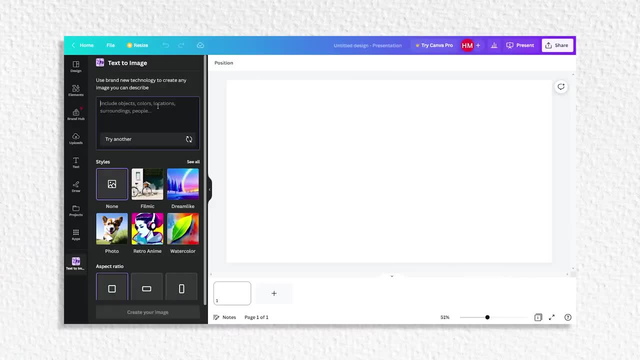 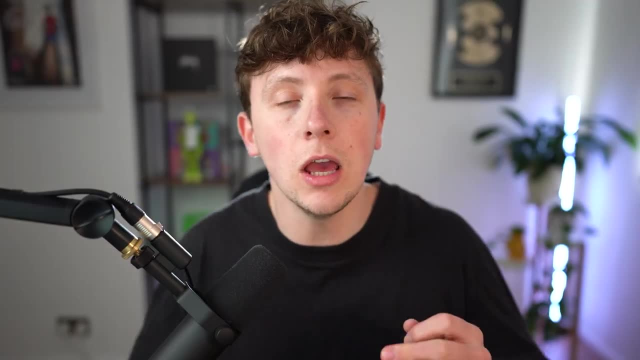 capabilities. We can essentially come on over to this. We can type in what sort of imagery we want. For example, maybe we want pink donuts on a pink background. then we can enter that into Canva AI. Obviously, you've probably taken photos of your donuts, if you have a donut shop. 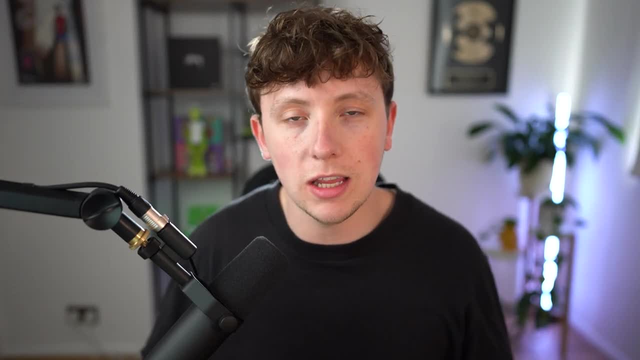 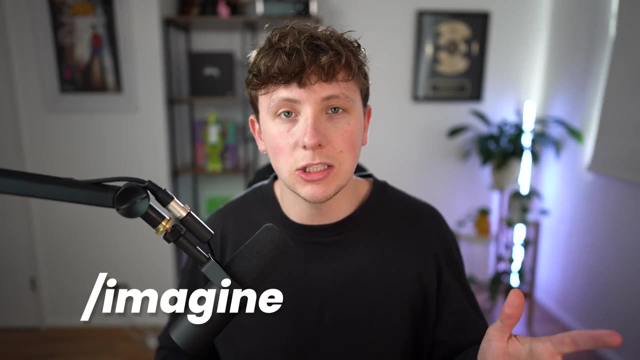 so you can use that as well. but if you did want to create them artificially, this is a great option. Now also, you have the likes of Midjourney, where you can type in different prompts. You type slash. imagine pink donuts. 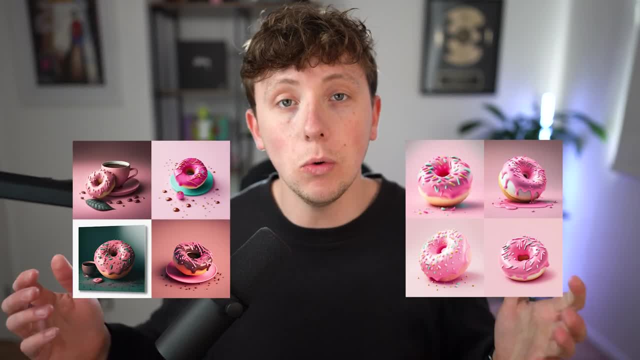 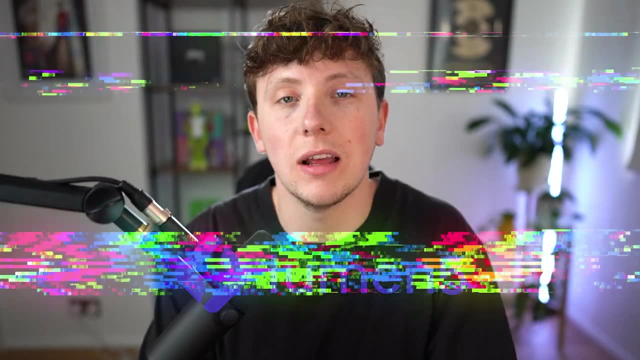 then it's going to spit out some amazing AI-generated donuts that we could also use on our social media. If I wanted to create video-based content, I could come on over to Lumen5.. Now Lumen5 is going to allow me to generate video content based on prompts and based on what I 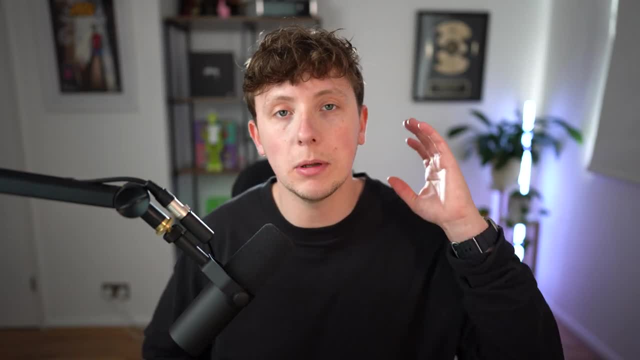 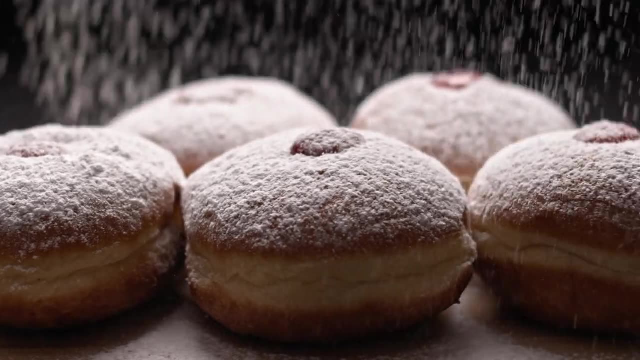 input into the system. Let's say, for a special ad. I'm going to be running a 50% discount, so I want to show a picture of a happy customer that is going into the store, tapping their card and receiving a box of delicious donuts. I can type that into Lumen5 and it's going to spit out. 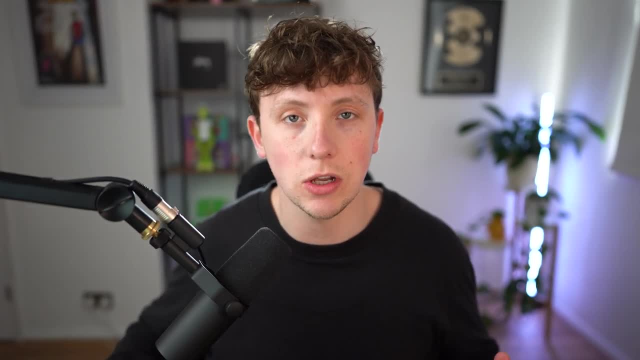 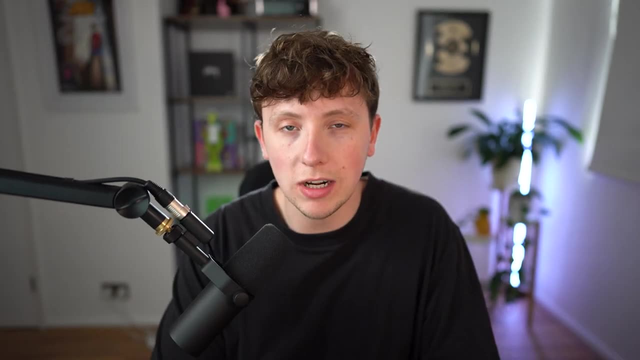 a video piece of content, where I can then add captions and change different titles, that I can then use as a video format on my Instagram, TikTok, wherever I want to use it When it comes to creating content from scratch, without the help of any pre-recorded videos or photography. 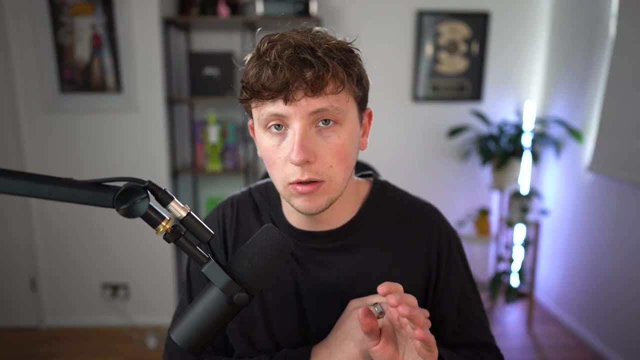 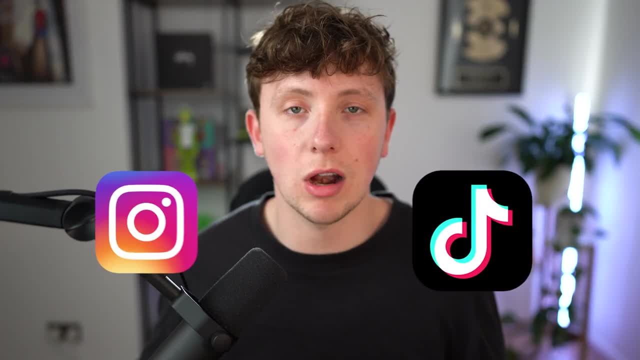 scratch. It's a great tool to create content from scratch. If I do take videos in the store and I upload them to TikTok or Instagram, I'm going to want to be able to add captions, These little words that come up on the screen as I'm talking right now. you can start to read along. 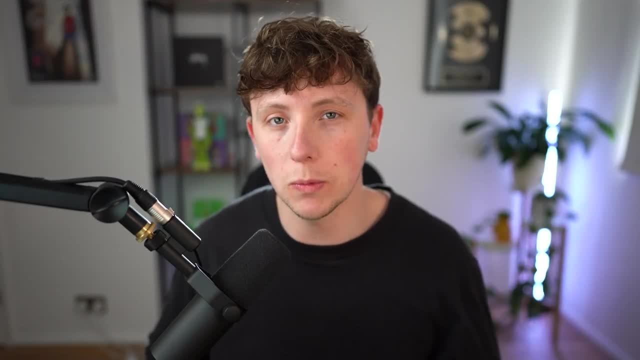 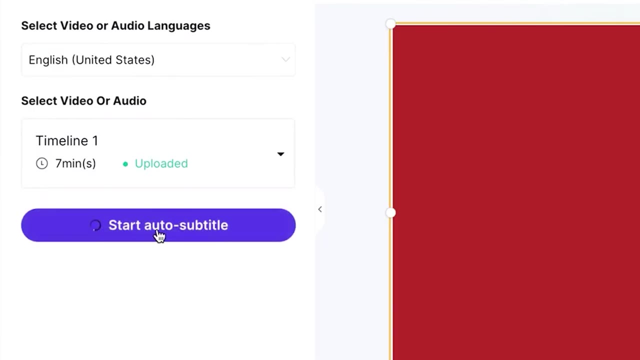 without having the volume on. These are super crucial when it comes to posting short form content. I'm going to show you exactly how you can do that using AI. There's a platform called mediaio. What you can do: you can upload your content onto that and AI will automatically add. 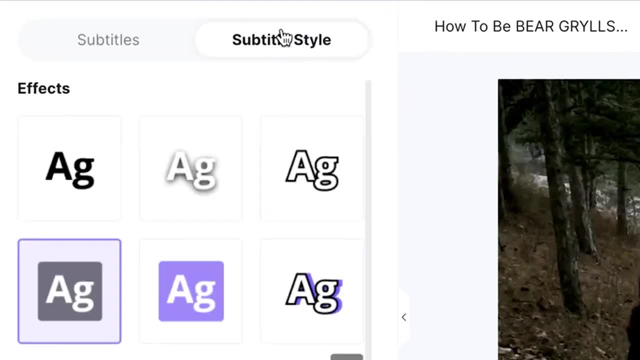 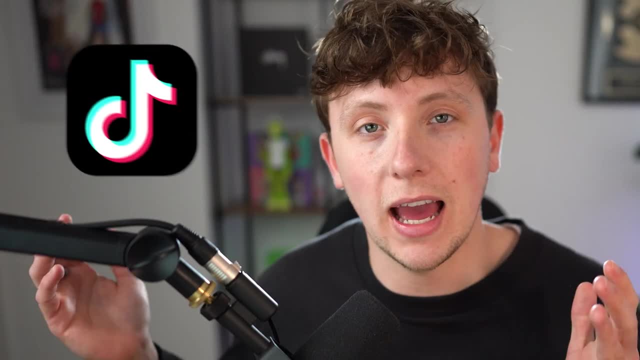 captions to your video. You can choose what font, you can choose what color, and you can choose what style and design you like as well. You can then move that text around the video, so it's perfect for you. Then you can use that on your TikTok and. 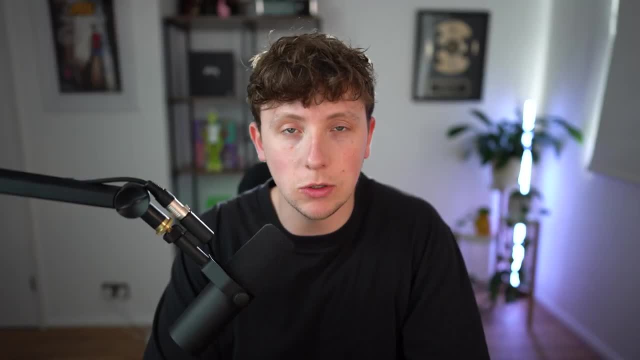 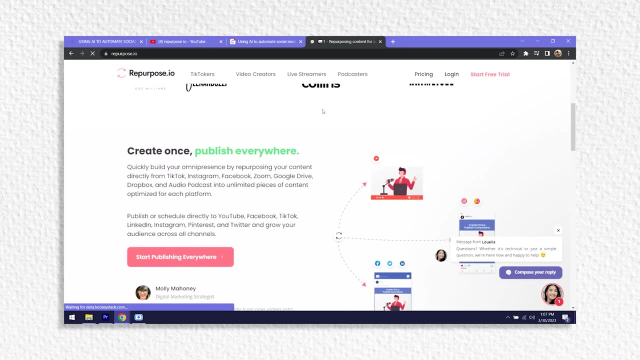 Instagram. This is obviously going to save you so much time. When it comes to repurposing your content. I would recommend going to repurposeio. Repurposeio automatically repurposes your content whenever you upload it onto a certain channel. Let's say you've made a YouTube video and you 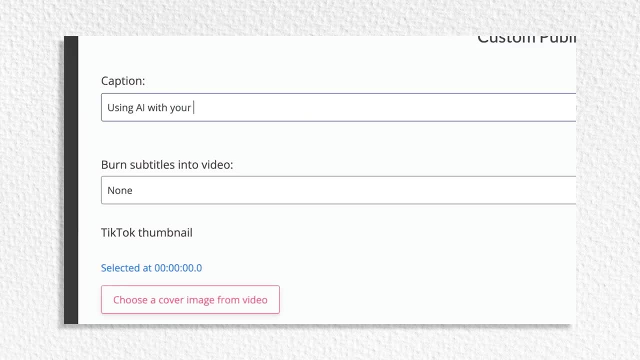 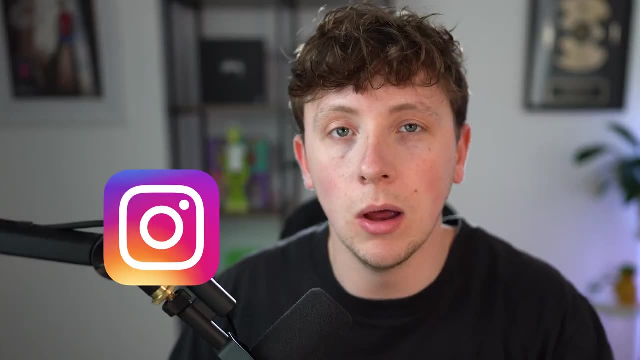 uploaded that onto YouTube. If you've plugged your channel into repurposeio, what it's going to be able to do is take that content from YouTube and then make it work on TikTok or make it work on Instagram, Whatever you have set it to do. That is just another way how you can automate your content creation using AI. 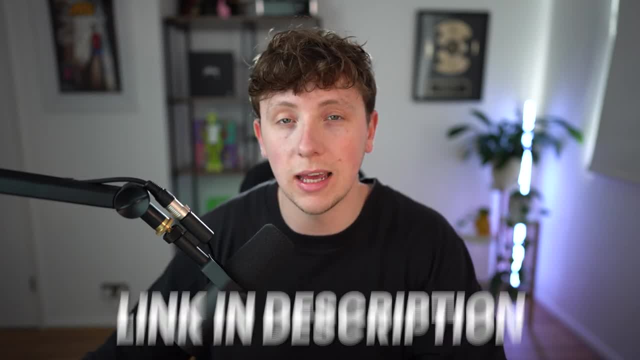 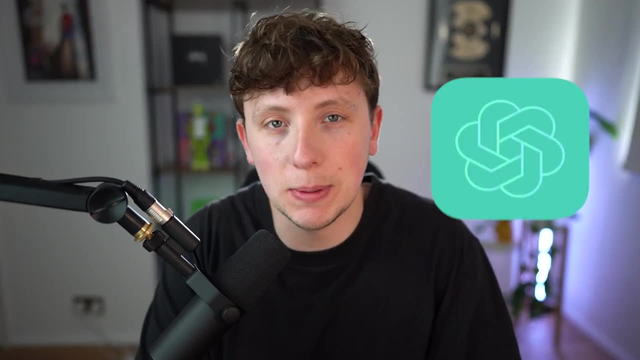 I'm going to leave all the links down below in the description for all the tools I talked about today. Once I have everything and I've got all my content ready to go, I obviously need to create captions for my content. For this, we're going to use ChatGPT. ChatGPT gives us so many different 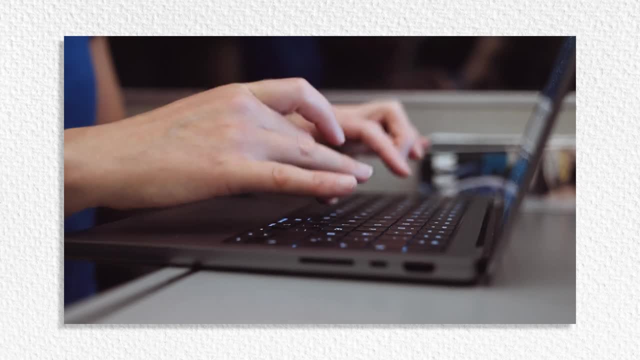 options for this. We can ask it to create us captions that are funny, create us captions that are in a bullet point list. We can also feed in data as well. We can say, hey look, we have a doughnut shop, We have a 50%. We can say, hey look, we have a doughnut shop, We have a 50%. 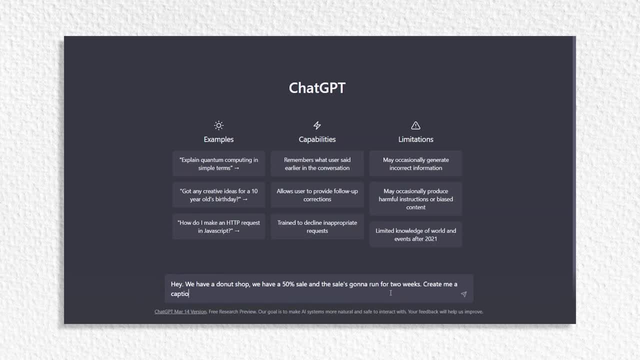 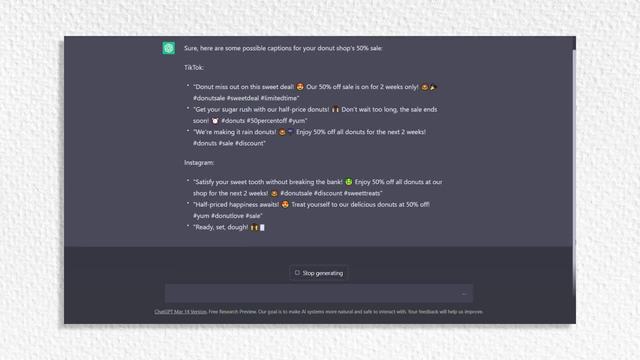 The sale is going to run for two weeks. Create me a caption for TikTok, or create me a caption for Instagram. ChatGPT is then going to spit out a ton of different caption ideas for us that we can then copy and play with Once we have all of our content created. 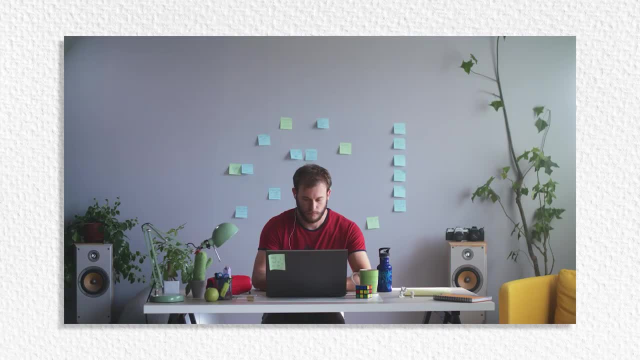 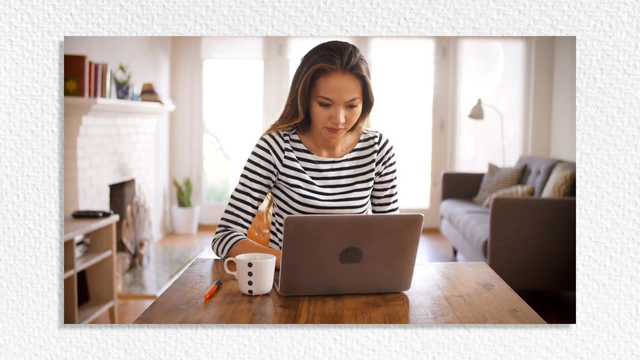 we are ready to go. We now want to schedule our posts. Content scheduling is going to take the pressure away from us to having to log into our socials every day just to manually upload all of our posts and imagery. We can now schedule and have everything done for us. We can schedule one. 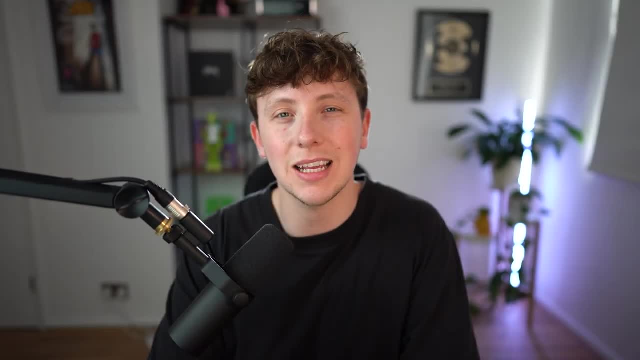 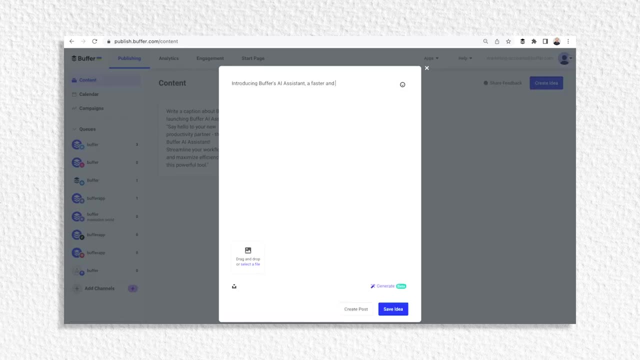 or two times a month. We can schedule one or two times a month. We can schedule one or two times a month and have posts going out every single day. still, Let's get them automatically scheduled for us. There is an AI called Buffer. What Buffer does? it allows us to schedule our content across these. 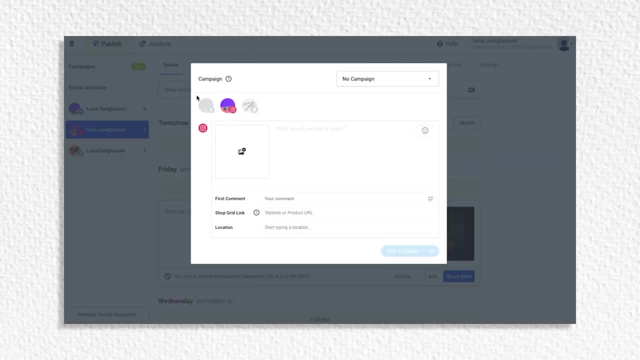 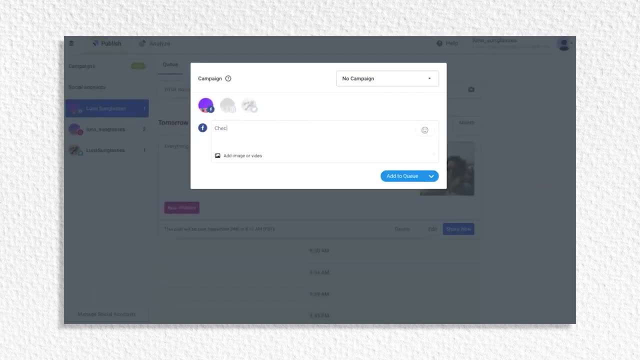 different platforms and completely automate our posting. Buffer is such a good all-round social media tool. It allows us to schedule all of our content. It allows us to create content and come up with content ideas for us. We can basically just plan everything when it comes to our social. 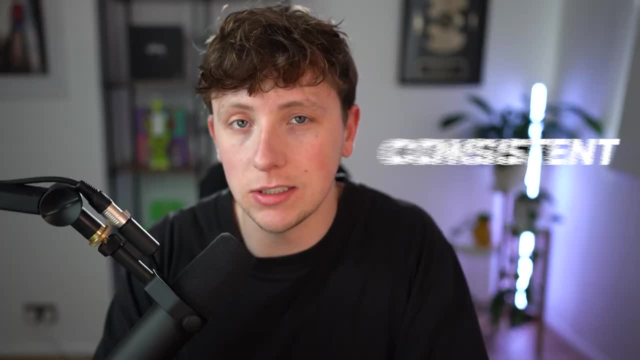 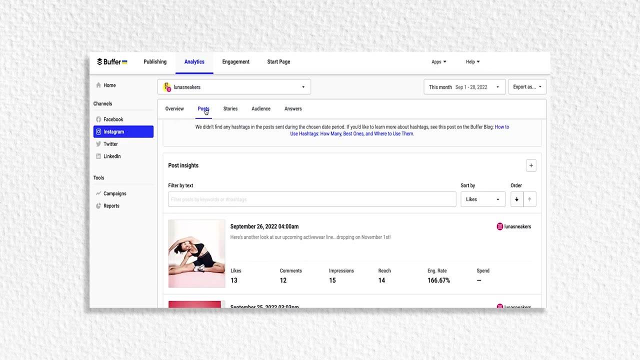 media on this one platform. The key here for us is to have a consistent posting schedule, And then we also need to be able to track and analyze our results of our social media posts once we have them set up and running. So you can actually do this on Buffer, too. They do. 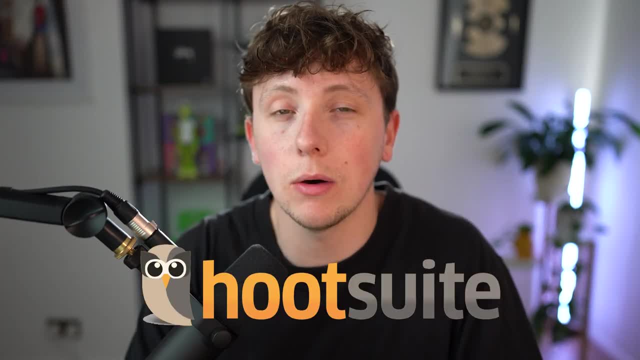 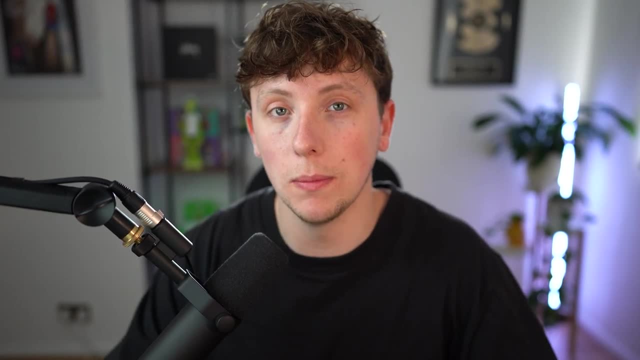 have an option for you to do that. There is also a platform called Hootsuite. Now Hootsuite has been running for years. A lot of people are using them, but they also have AI integrated into their platform now as well, So Hootsuite is going to allow you to track all. 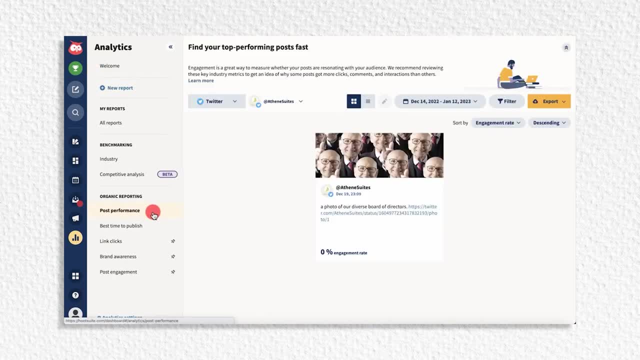 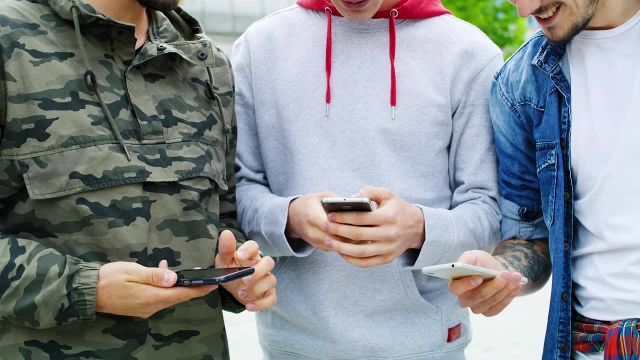 your analytics, see how well your posts are doing, see what levels of engagement you're getting on what posts as well, and then see what channels are working the best for you too. You see it all the time. A lot of people get excited on social media. They think that they just have to constantly post. 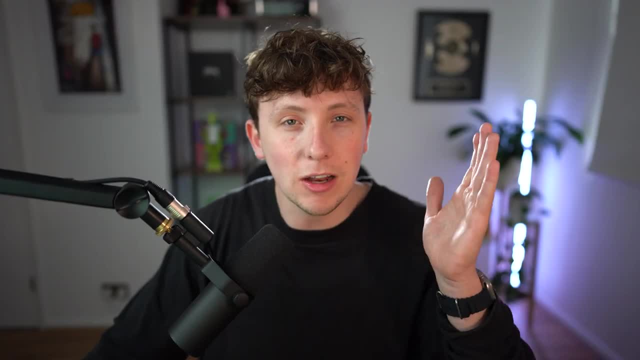 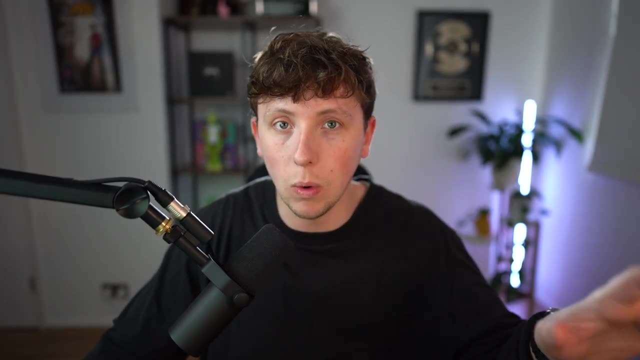 on every single platform, which, yes, I somewhat agree with. But if there is a platform that is absolutely killing it, like TikTok for example, you need to be allocating 60, 70% of your time to that one platform and then just keeping the other platforms active. So there's always going. 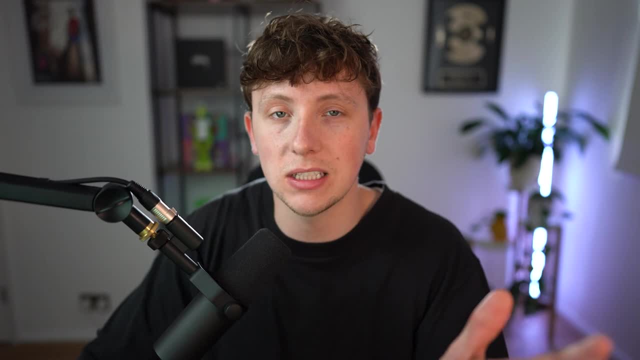 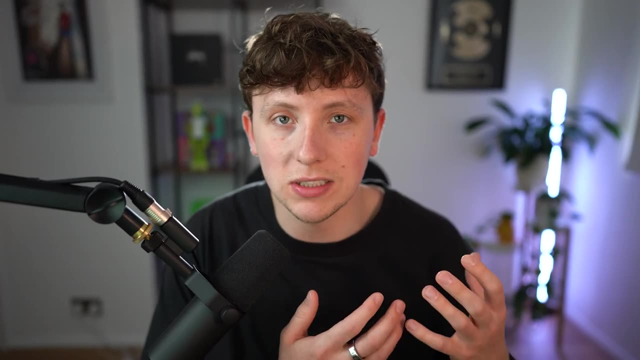 to be that one winner for you guys, And it all depends on your different business. If I'm selling donuts and my demographic of customers is younger people in their 20s, then I'm going to want to be on TikTok because that's where my audience is. 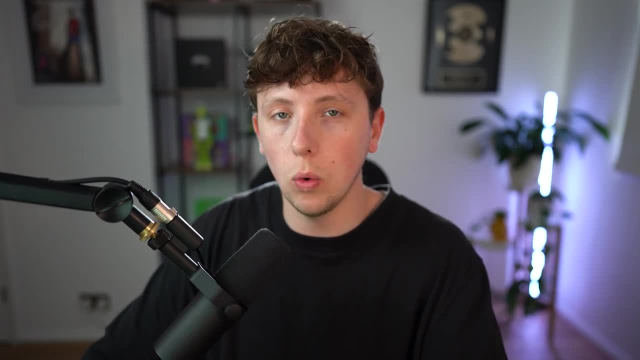 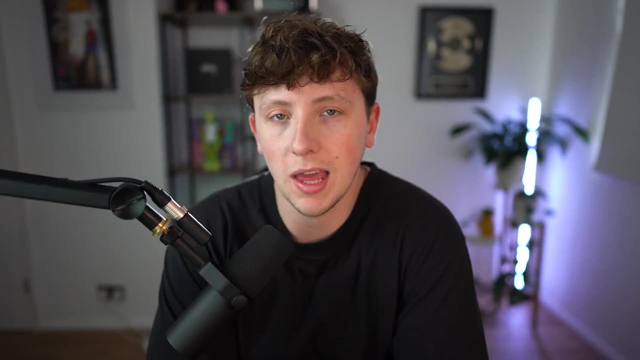 So you do have to understand that, when it comes to social media, not everyone is on all the platforms. You need to really decide where your demographic is and where you're going to get the best value for your time. It doesn't just stop there, though, Once we have everything set up. 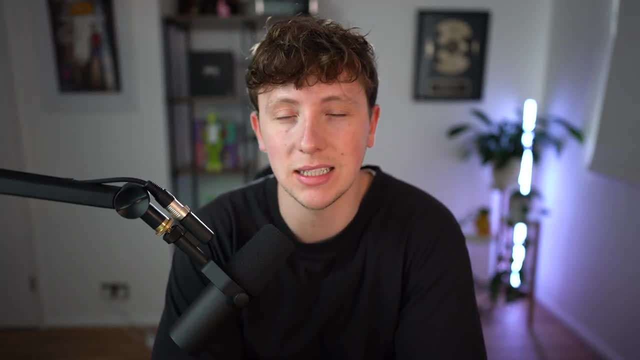 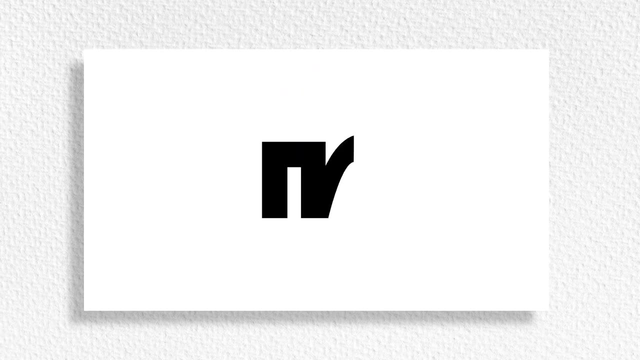 we have our content ready. we have our posting schedule. we're now tracking our analytics and data. We also want to use some AI to actually manage our community, So we have a platform called ManyChat. Now, what ManyChat is is a chat bot that you can plug into your Instagram.